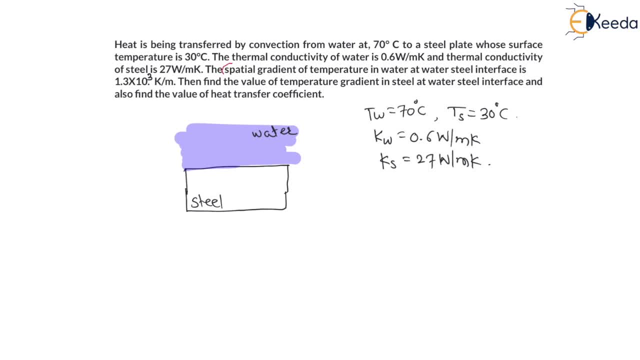 Now, my dear students, let us understand this spatial gradient. Spatial gradient is nothing but temperature gradient. Spatial gradient is nothing but off-temperature. It is written off-temperature Means it is a temperature gradient That is dt by dy. 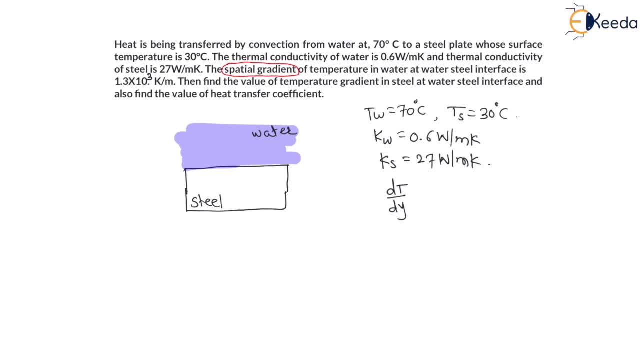 Temperature gradient is dt by dy with respect to y, Because here it is a height y See with respect to y, this spatial gradient will change. Right Now this dt by dy is given Again you can see from the unit Kelvin per meter. Kelvin is temperature dt, Meter is distance dy. Therefore it is dt by dy. 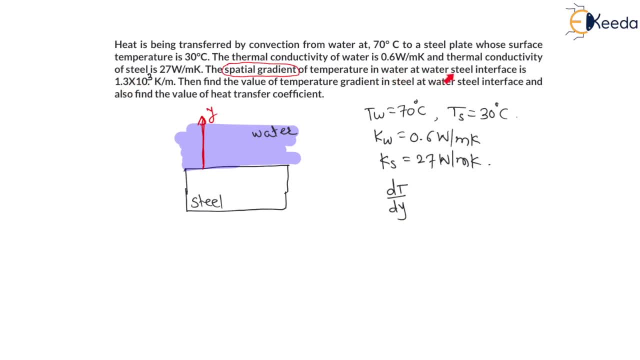 For it is given in water at water-steel interface. Now here at this interface, at this interface in water right, they have provided as 1.3 into 10 to the power, 3 Kelvin per meter. Then find the value of temperature gradient in steel at water-steel interface. At the same interface, we have to find temperature gradient in steel, That is dt by dy. 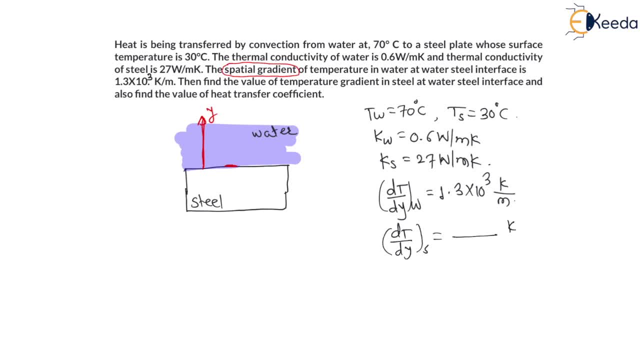 In steel. we have to find Same unit, Kelvin per meter. We have to find in same unit, Right Then, and also find the value of heat transfer coefficient. Now, for this water there will be a convective heat transfer coefficient, H. Therefore this H of water we have to find Convective heat transfer coefficient is Watt per meter square Kelvin. 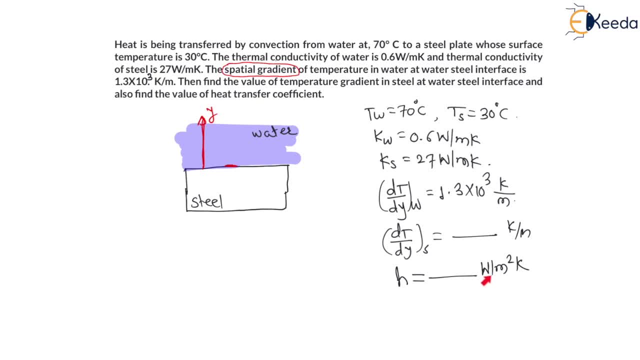 So we will find in this standard SI unit Watt per meter square Kelvin. Now here, as temperature of water is more than temperature of steel. therefore, heat is flowing from water to steel. Now let us understand the direction of heat flow. Let us say the temperature of water. at this location, temperature of water is 70 degree Celsius. 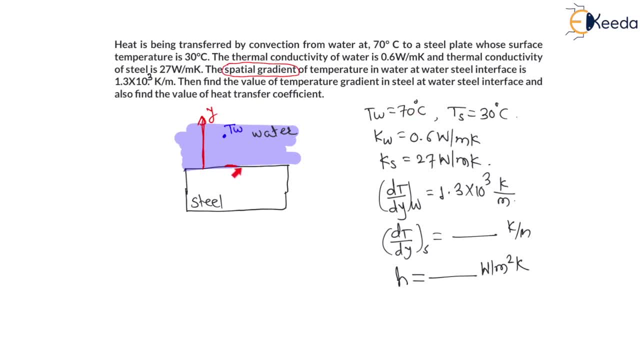 It is given here, And steel temperature is 30 degree Celsius at this interface. Therefore this surface temperature of steel is Tf Right Now. definitely in water there will be a convection: heat transfer Means from this temperature of water to this temperature of steel. there will be a convection. 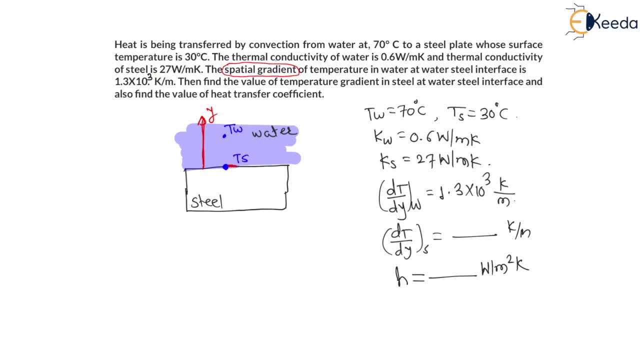 Therefore, very first mode of heat transfer Between water and steel surface is convection. This will be convection Right And, my dear students, the first layer of water in contact with steel will be under no slip condition. We can say this first layer of water molecules in contact with this steel is under no slip condition. 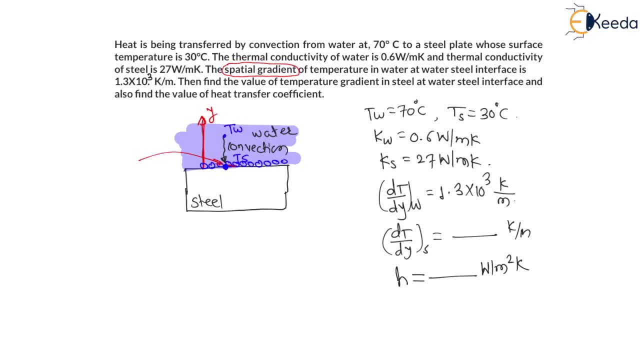 That's why in this first layer there will be a conduction. I can say, between this first layer and this steel surface there will be a conduction, Conduction in water, In water, This will be the conduction in water. 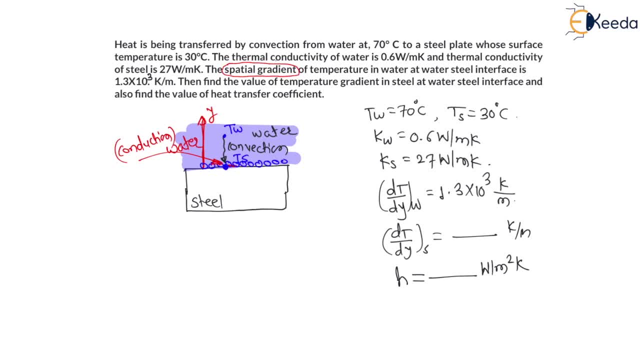 And after this conduction, inside this steel, there will be a conduction again. As steel is a solid surface, there will be a conduction in steel. This conduction is in steel And, my dear students, we know that for steady state condition, for steady state condition, steady state condition, we can say the heat transfer at each and every location is same. 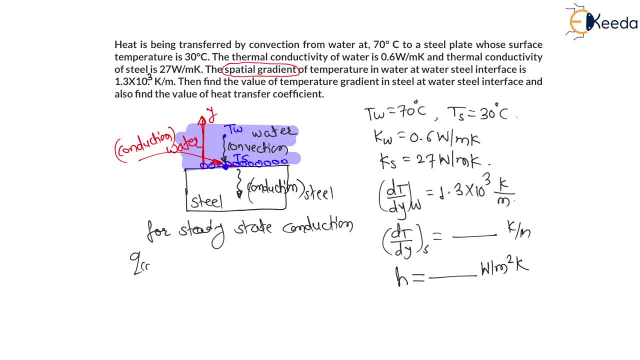 Means this heat transfer by convection. Heat transfer by convection inside this water is equal to heat transfer by conduction- Heat transfer by conduction inside water at water-steel interface And is equal to heat transfer by conduction at in steel inside this steel. 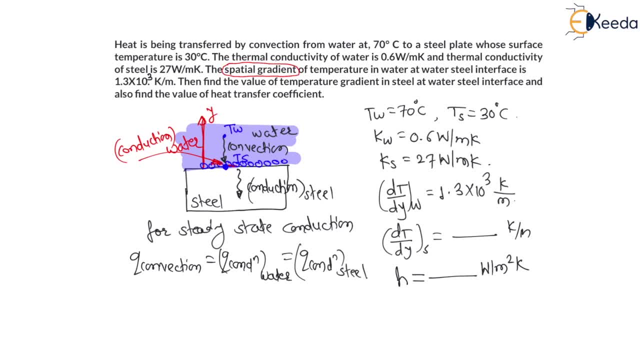 Right. This equation we can write for steady state condition. Right. If I mention somewhere glass, it is not a glass, It is a water and steel interface, Right? So make a note that Now let us write down this formula. 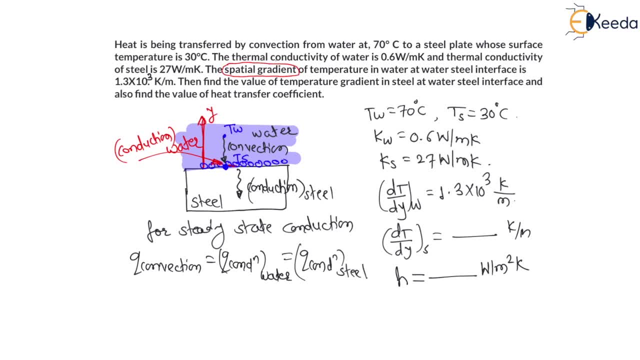 Now here. I will delete the question so that I will get sufficient space for the solution. Right Now. my dear students, here they are saying: the convection heat transfer inside this water is equal to conduction. heat transfer in this water is equal to conduction heat transfer in the steel. 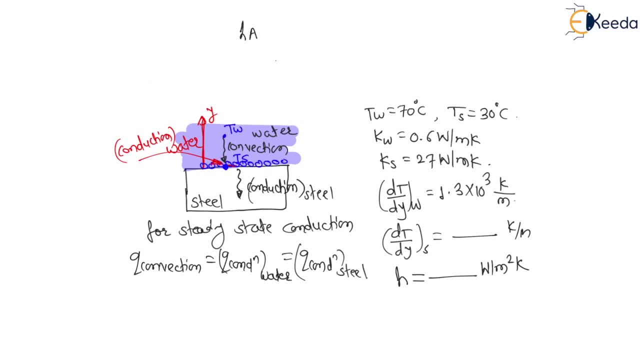 Therefore we can write: Convection heat transfer is Ha. Convection heat transfer is convective heat transfer coefficient Eh into area, Into temperature of water minus temperature of steel, is equal to Now. conduction heat transfer is Ka dT by dx. 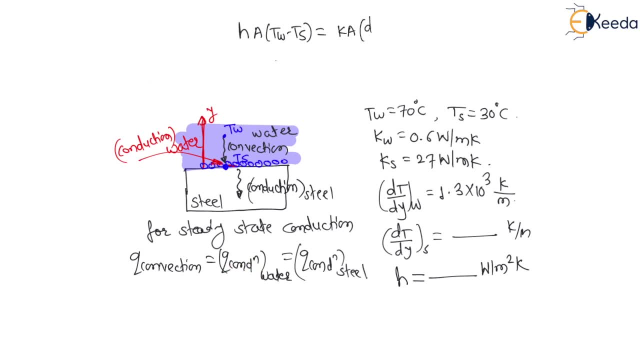 As per Fourier law of conduction, it is Ka, dT by dx, but here along y direction. Therefore we can write dT by dy. First of all, we will write: for water is equal to, then for steel: Ka along y direction, dT by dy for steel. 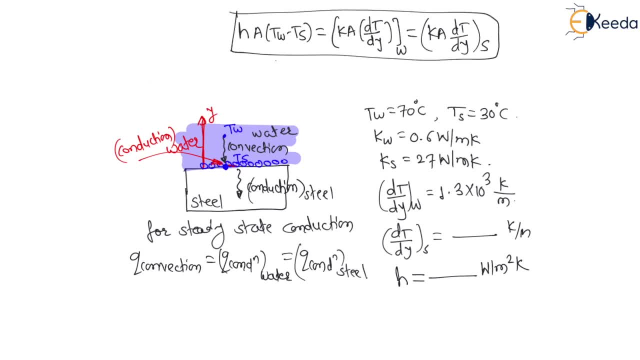 Right, This is how the expression can be written. This is how we can write the expression. Now, here you can find this. for convection, the area is area of contact between the water and steel surface, And for conduction, the area is perpendicular area to the direction of heat flow. 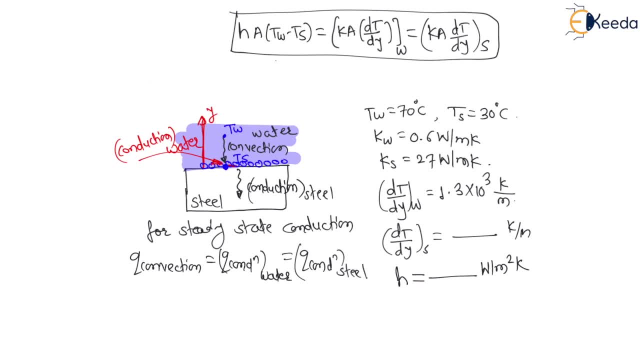 Now heat is flowing along y direction. Therefore, for this y direction, if I consider perpendicular area, the area will look like this: Right See, this top area is perpendicular area, as well as this top area is the exposed area between water and steel. 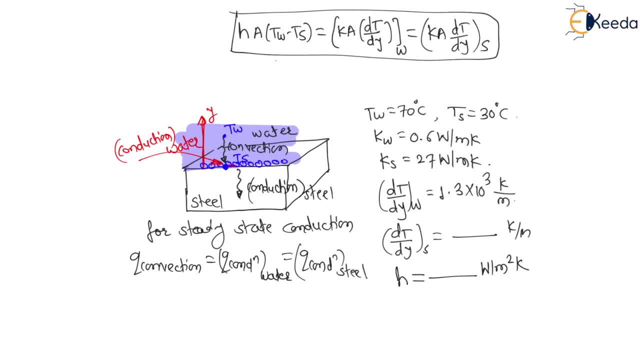 That's why we can say here: this area, this exposed area, is same for both water and steel And steel interface, as well as for direction of heat flow perpendicular to the direction of heat flow. Therefore, this conduction area and convection area are same. 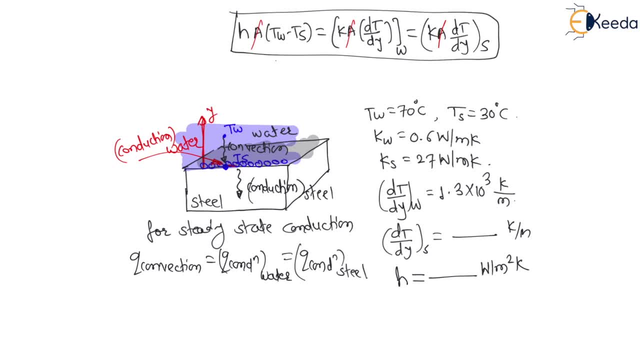 Therefore they will get cancelled from both side. Therefore the equation becomes: Eh into: temperature of water minus temperature of steel is equal to Ka dT by dy of water is equal to Ka dT by dy of steel. This is how the expression can be written. 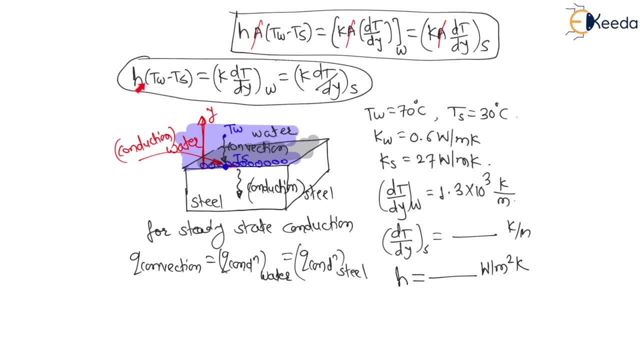 Right Now, let us put the values Here. Eh is unknown. We can find Here dT by dy of steel is unknown. These values we can find with this equation Right Now. I will delete this diagram so that we will get sufficient space for the solution. 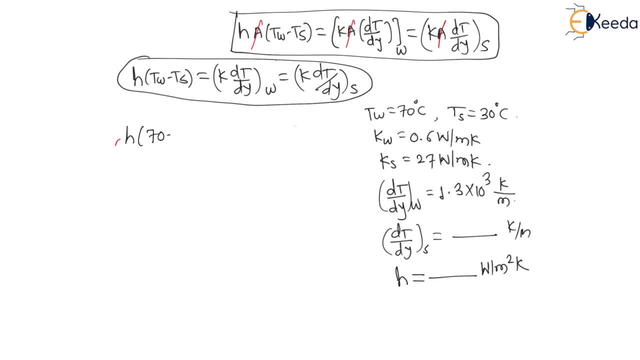 Therefore here equation becomes Eh into: temperature of water is 70 minus. temperature of steel is 30 is equal to thermal conductivity of water is 0.6 into dT by dy of water. Here all the values are given: Thermal conductivity of water, thermal conductivity of steel, dT by dy of water. 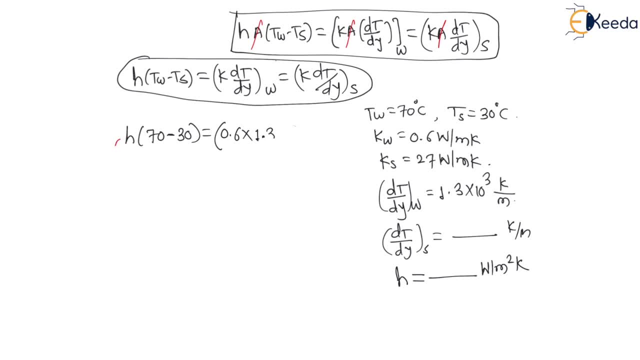 Right. Therefore temperature gradient of water 1.3 into 10 to the power 3 is equal to thermal conductivity of steel is 27 into dT by dy in steel. Right Now, if I equate second and third equation then I will get temperature gradient in steel. 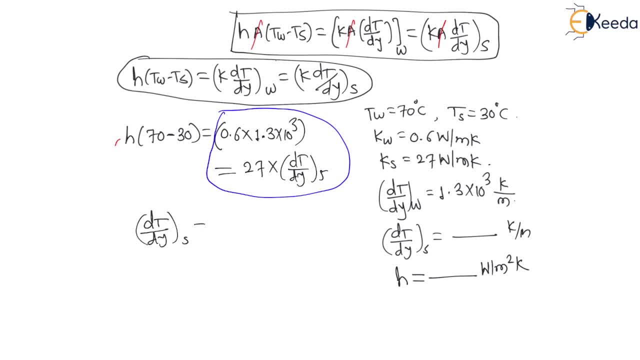 So let us find this dT by dy in steel. Comment me this answer. This answer will be in Kelvin per meter And if I equate first and second expression, Then I will get the convective heat transfer coefficient, the Eh value. 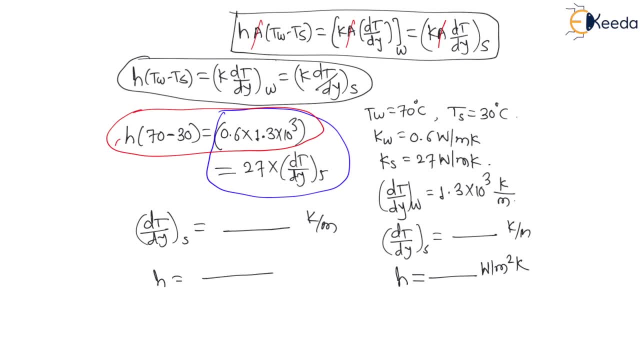 Right, And let us find this Eh value And this answer will be in Watt per meter square Kelvin, And let us put your comment here Then. first answer, that is dT. by dy of steel you will find as 28.889 Kelvin per meter.